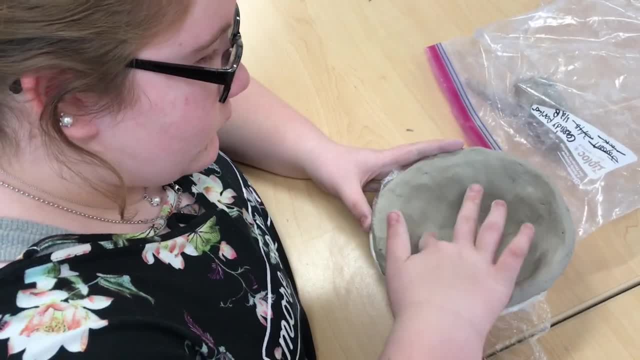 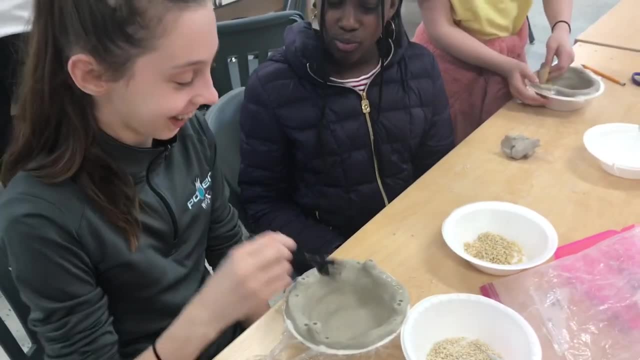 Really squishy Whoa Reese. how did you get your bowl so smooth? Well, first I took a board and I started scoring my bowl, And then I smoothed it out. Also, when you're done with that, you can use a sponge. 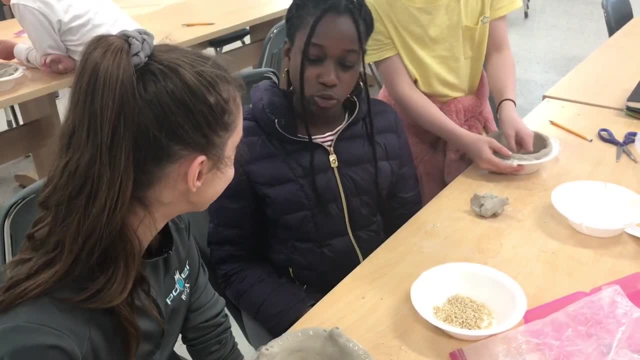 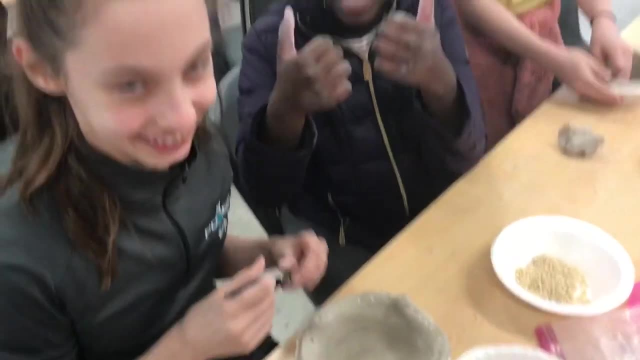 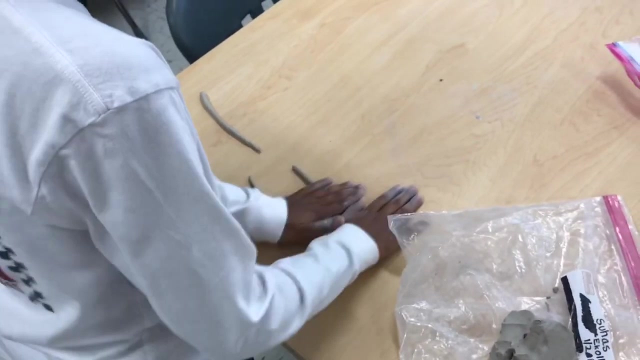 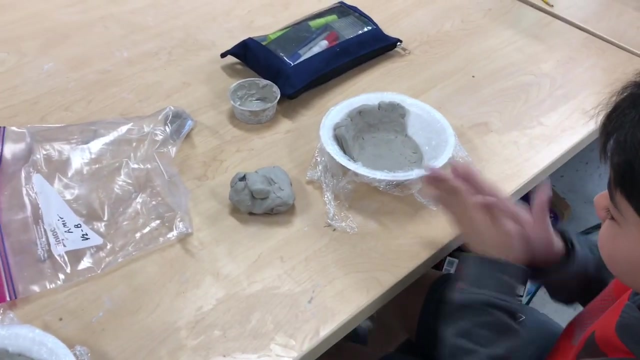 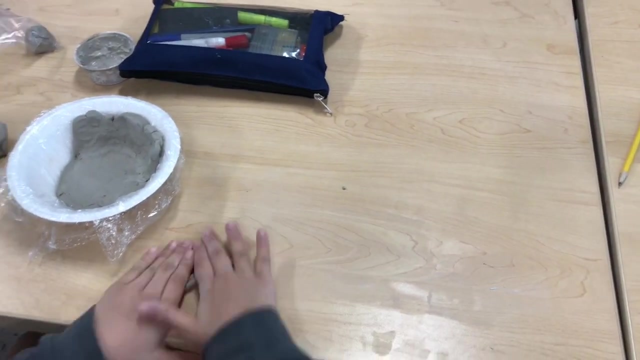 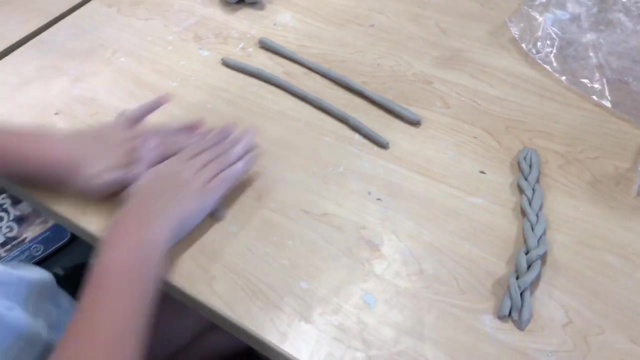 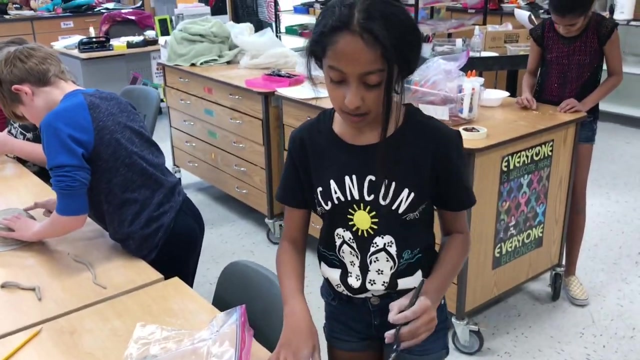 Wait, You have to use a damp sponge, and it has to not be too wet so it doesn't ruin your bowl. Yes, and then you'll get a super smooth bowl. It doesn't stick together automatically, so what you have to do to keep your pieces together is score it. 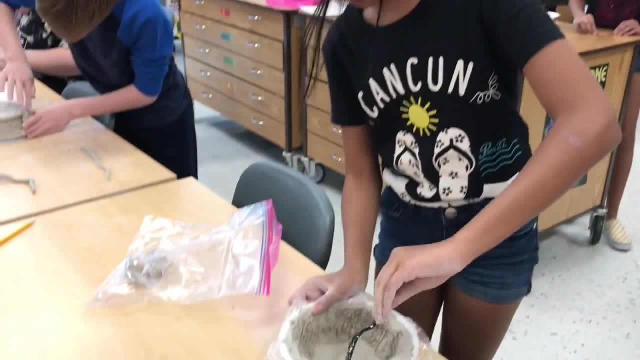 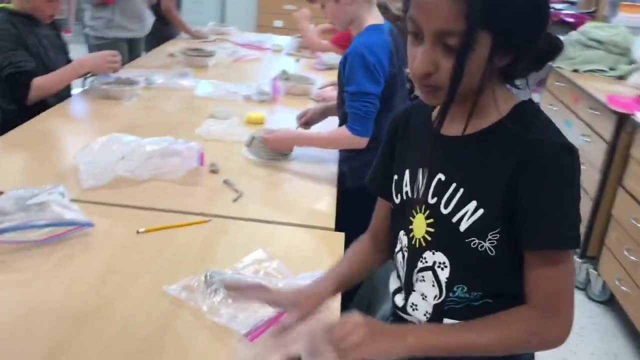 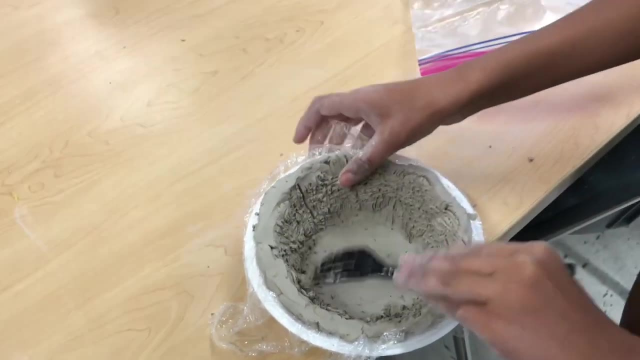 So I'm just using a fork right now to help it. What you're basically doing is just creating kind of like a velcro kind of thing and you're just throwing lines And you make them go into the sides, going vertically, And then when you're done with that and she's done it all around your bowl. 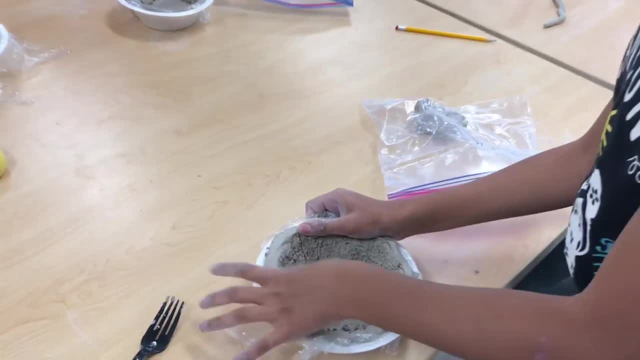 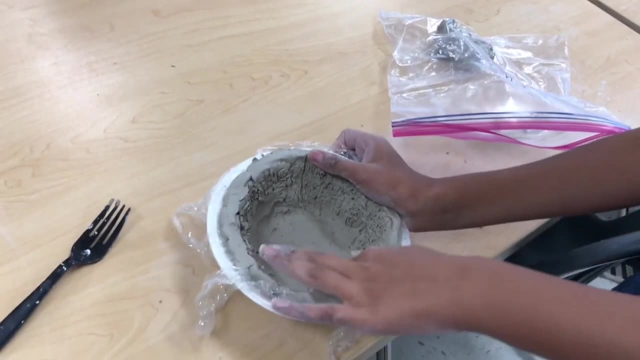 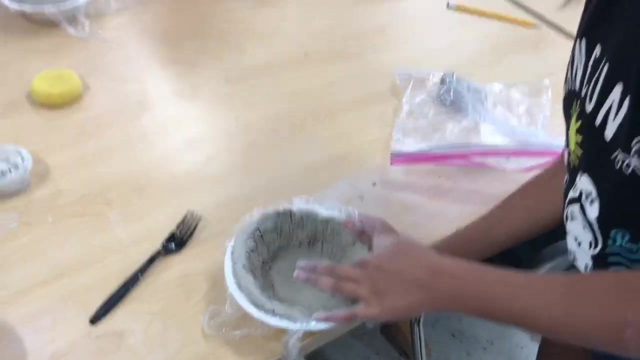 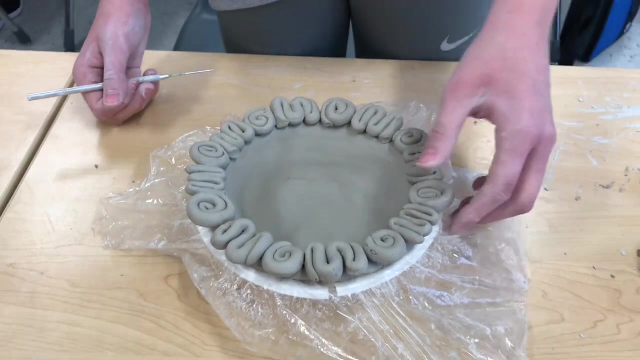 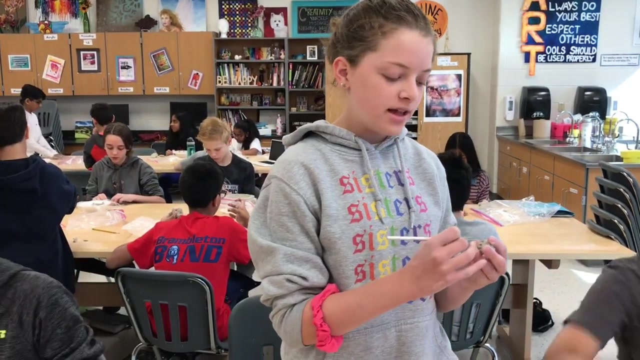 you have to score it like this and squeeze it out like that, And now they will actually stick and you don't have to worry about it just coming out. But to make them stick on I need to score and slip them. So first I'm going to take this needle tool or anything sharp like a pencil. 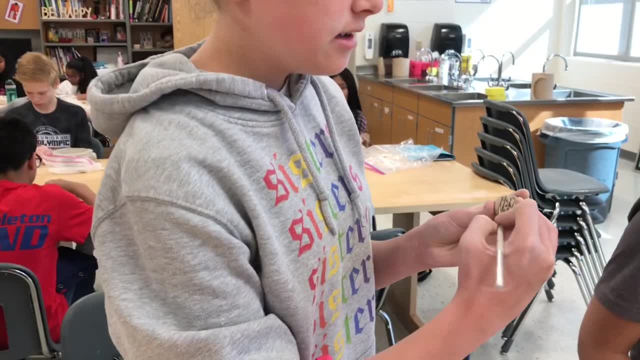 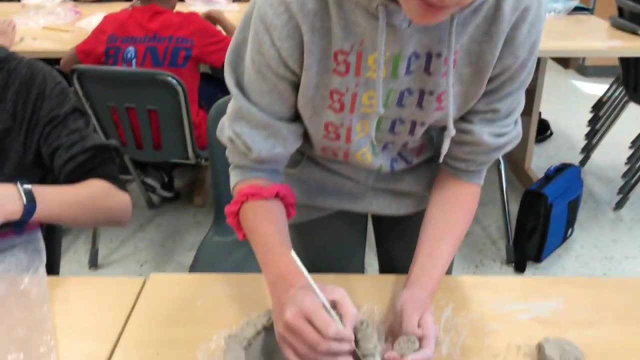 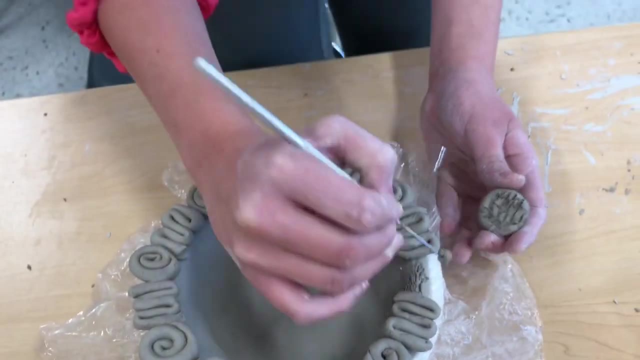 and just make lines like this, going horizontal and vertical, And then I'm going to do that on my bowl too, wherever I'm attaching it. Yes, I will Thank you. And then I'm going to take some slip which is just clay and water, just a little bit. 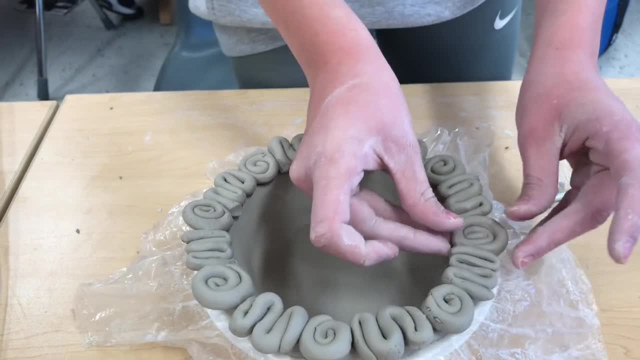 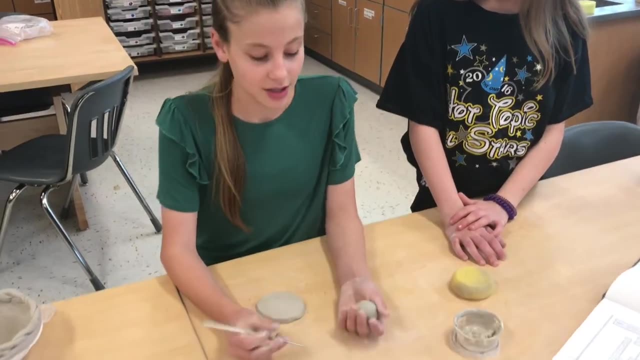 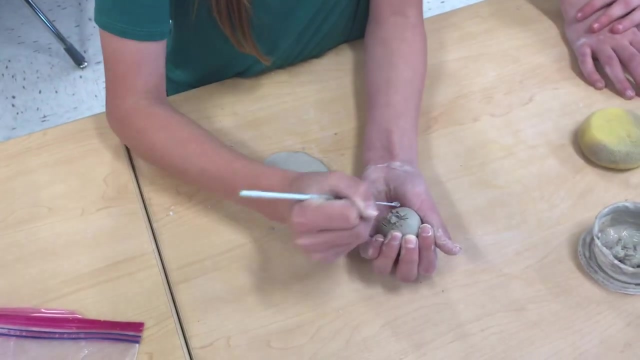 and then put that on there and then stick it on and wiggle it around and make sure that it is going to stay. Slip is made out of clay and water. If you want to score and slip, first use a tool to score your piece of clay. 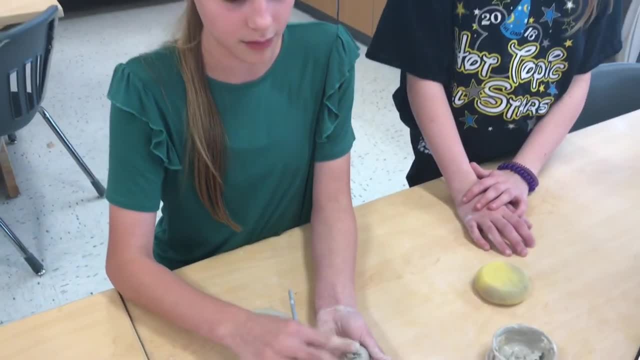 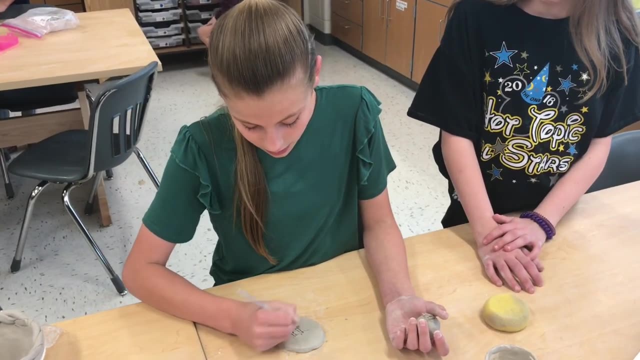 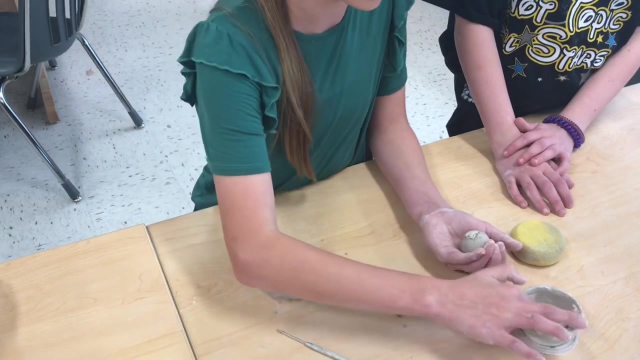 You can score it in different directions to make it easier. Next, score the piece that you're going to put the piece of clay on. Next, you can use some slip to make it easier to stick on for the piece And just press it on. 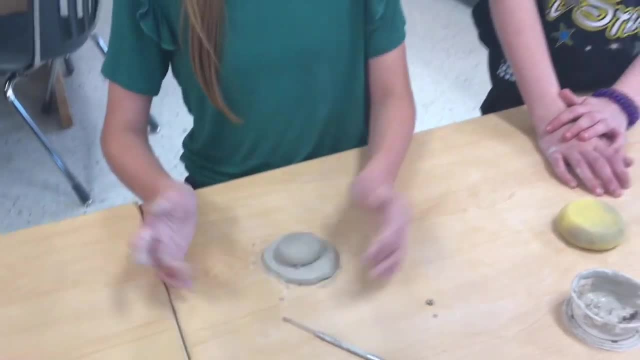 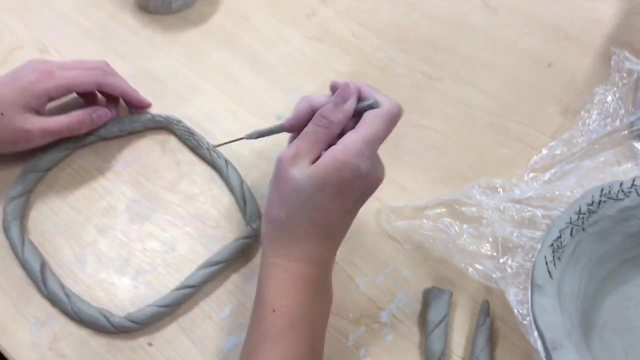 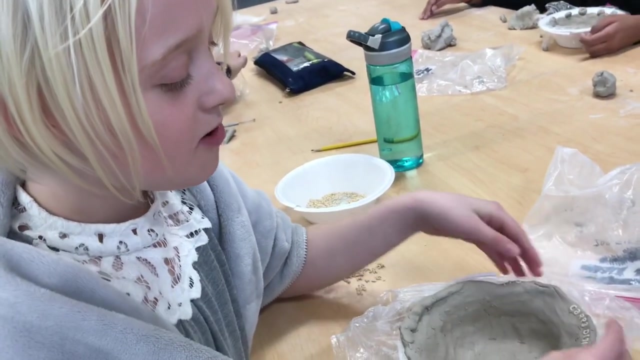 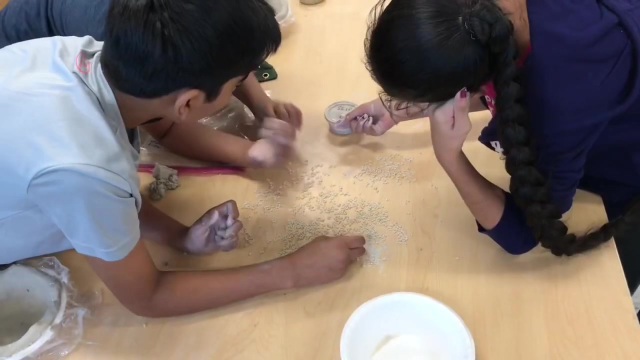 And if you can smooth it down. So I'm putting alphabet letters in my bowl. So when I bake it in the kiln it will blow away and it will disappear and it will leave an impression on your plate. Oh, This might be good. 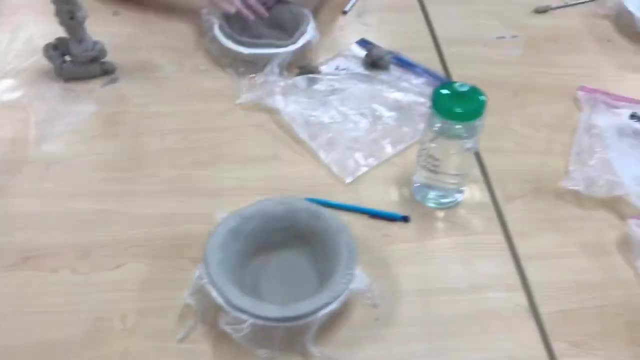 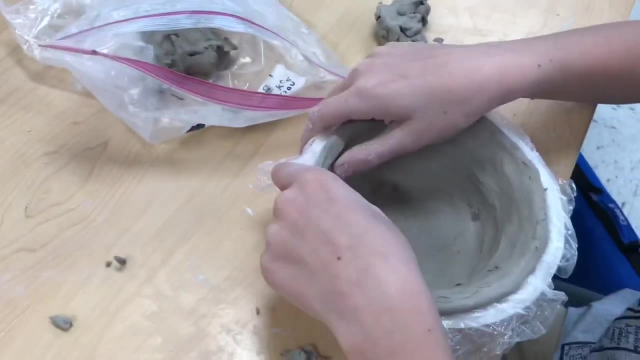 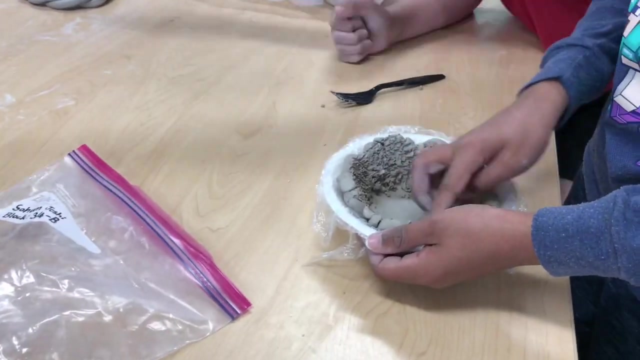 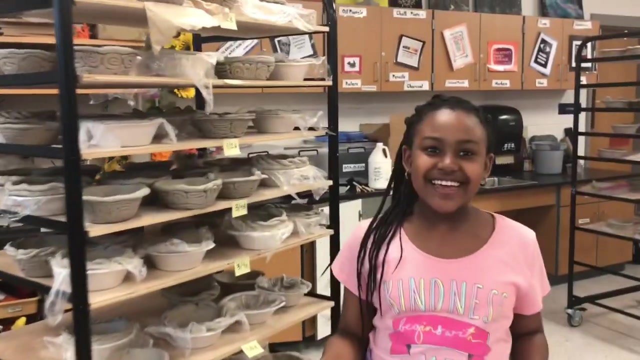 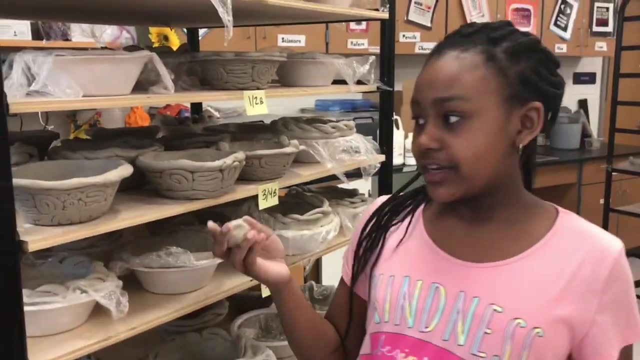 You have to eat, You have to eat, You have to eat. Greenware clay is clay that is able to work with and you can make a clay bowl out of Leather. hard is clay that still has some flexibility but is able to stay in its shape. 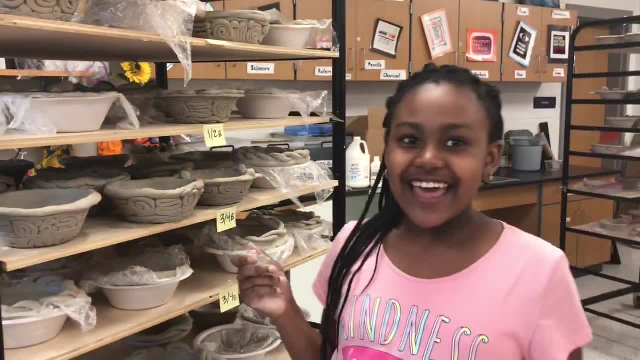 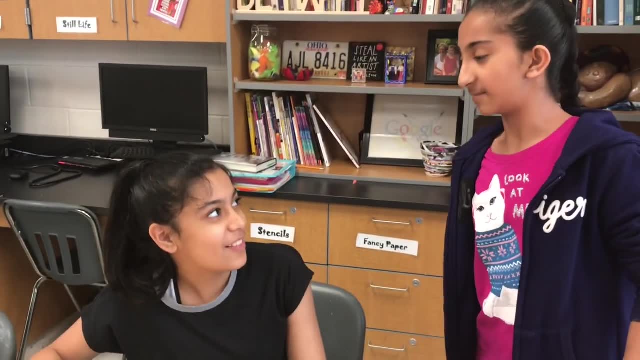 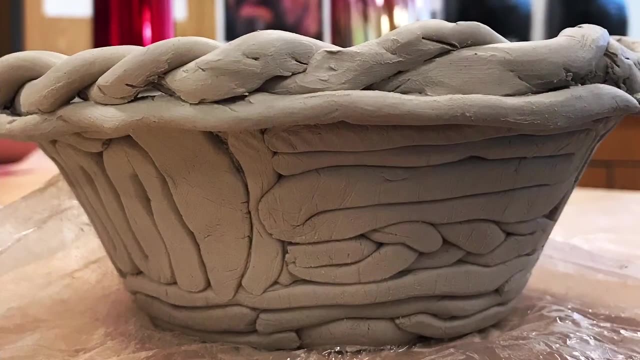 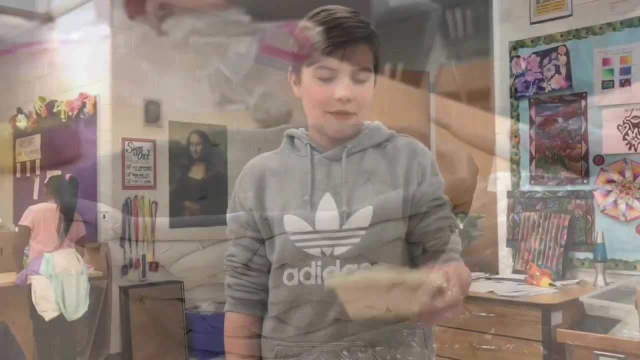 Bone-dry clay is basically dry clay that your teacher can put in the kiln. Hey, Harveen, what causes clay to permanently harden? Heat approximately 1,800 degrees from the counter After clay is fired. once it's called bisqueware, Then you're ready to glaze it. 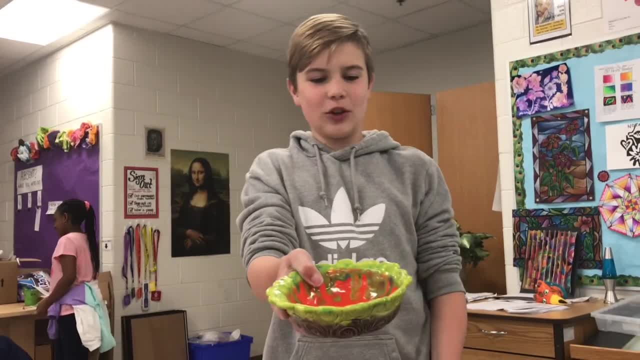 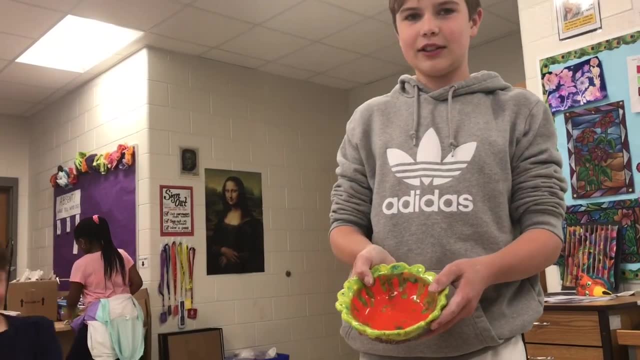 Once it's glazed, this is what it'll look like, and it's called glazeware. And once it's glazed, you fire it for a second time and then it'll look like this: